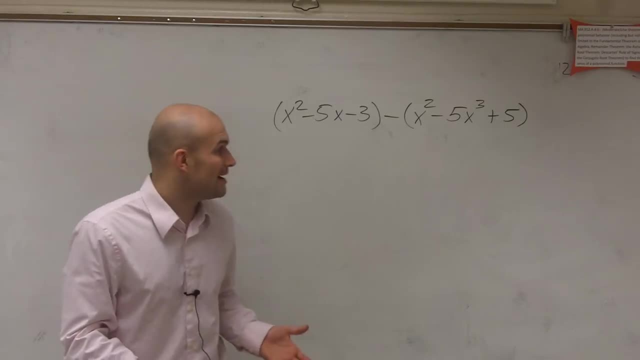 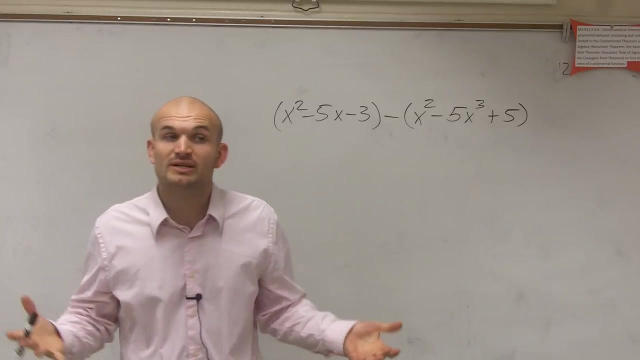 Okay, so what I like to do is show you how to subtract our polynomials, And when subtracting polynomials? I'm actually going to show you guys two different ways. First way, I'll show you the vertical method, just like we did with adding Adding. you're just going to 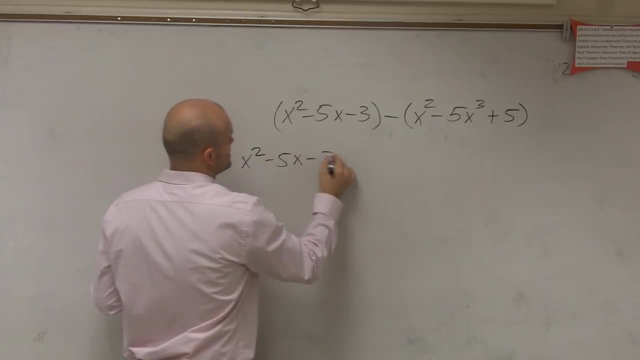 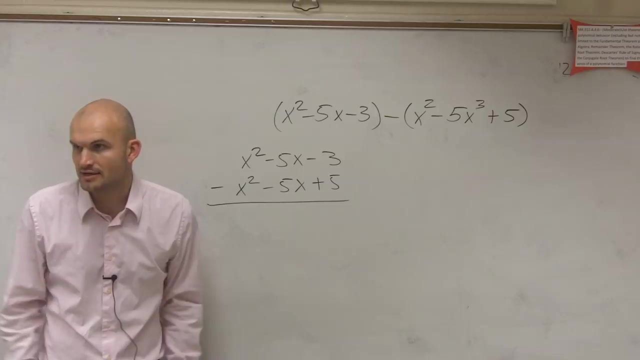 subtract. So you write x squared minus 5x minus 3 minus, and then you have x squared minus 5x plus 5.. Now I like this method because it's pretty simplistic. All you do is you take one equation and then you put it under the other equation and you subtract them. 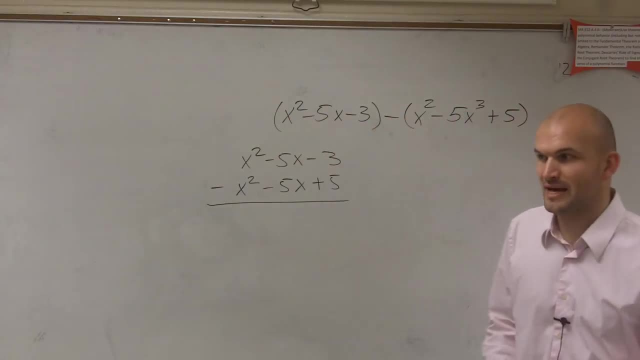 right. It's pretty straightforward, pretty basic. I don't like this method because a lot of times students make get mistakes and they forget that you're subtracting this whole bottom equation from the top, or this whole bottom polynomial from the top polynomial. 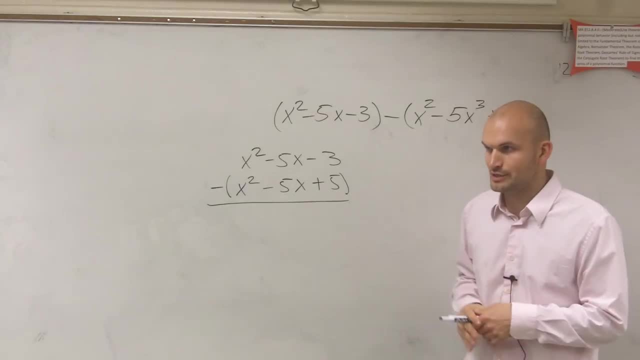 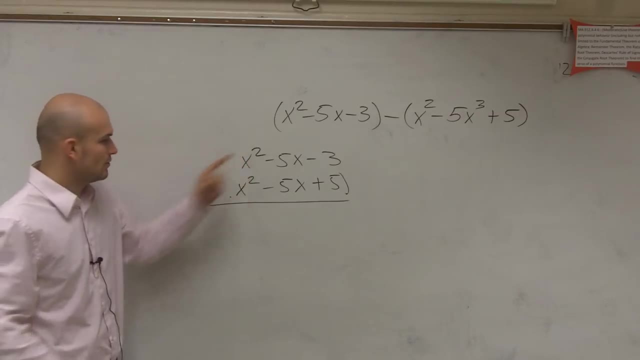 So when you do this, you have to kind of say it out loud to really make sure you're doing the correct operations. all right, So here's how I'm going to help you. So I have x squared minus x squared, which is going to be yes. Oh, that's not supposed to be a 3, I'm sorry. 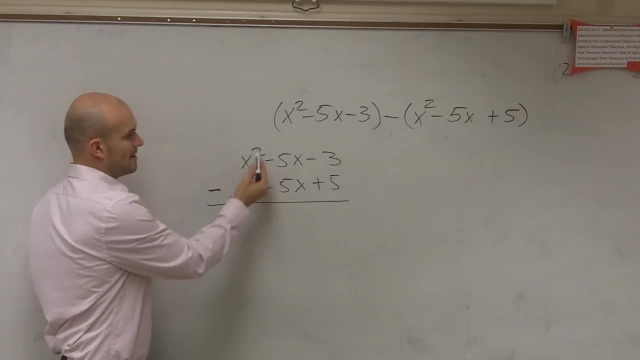 that's supposed to be an x, sorry, Okay. so x squared minus x squared is 0x squared 0 times x squared is just going to leave us with 0, right. So now? negative 5x minus negative 5x. Remember, those are double negatives, so it's going to be negative 5x minus negative. 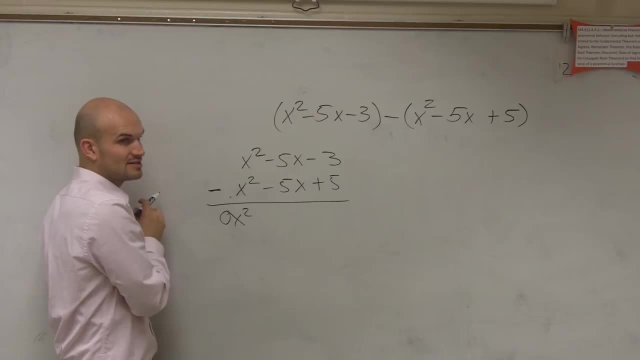 5x and it's going to turn to positive. so therefore, negative 5x plus 5x is going to leave us with 0x, and then we have negative 3 minus 5, which is just going to leave us. 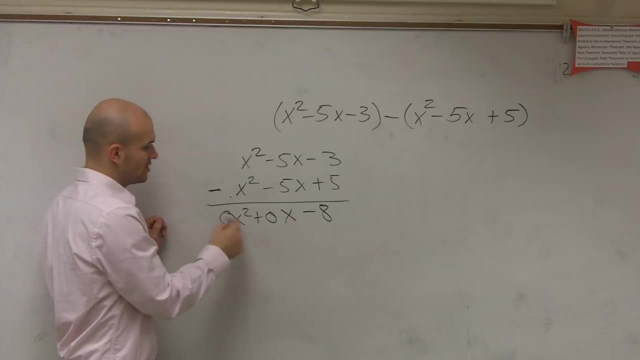 with a negative 8.. Well, obviously, like I said, these are all going to multiply to give you 0, therefore, your final answer is just going to be negative 8 in this example. okay, Cool. Now here's the other method that I think. 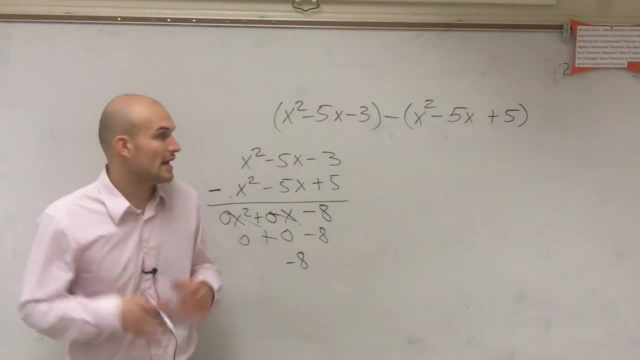 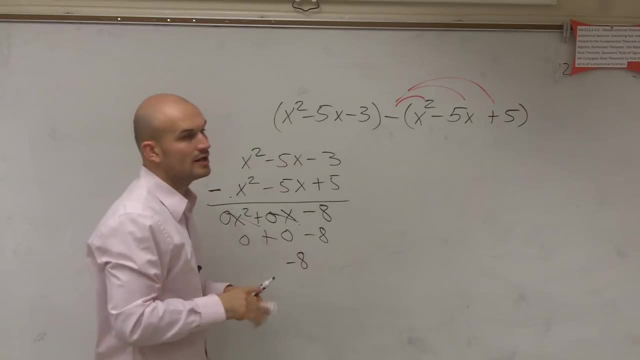 makes it a little bit easier, because I really don't like doing subtraction like this. What I prefer to do is apply the distributive property with your negative symbol. okay, Therefore, and then remember, remember, guys, when you first learned adding and subtracting numbers. 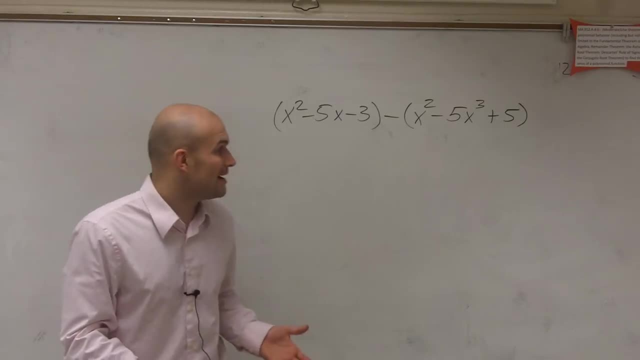 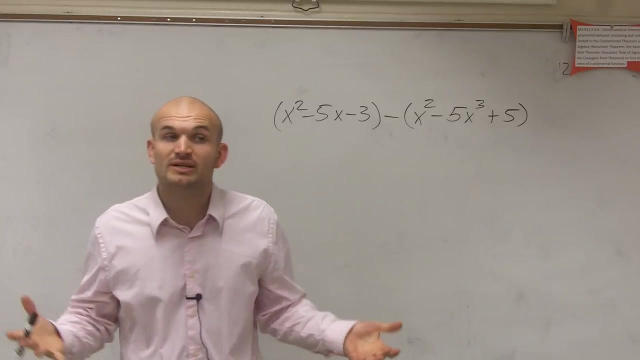 Okay, so what I like to do is show you how to subtract our polynomials, And when subtracting polynomials? I'm actually going to show you guys two different ways. First way, I'll show you the vertical method, just like we did with adding Adding. you're just going to 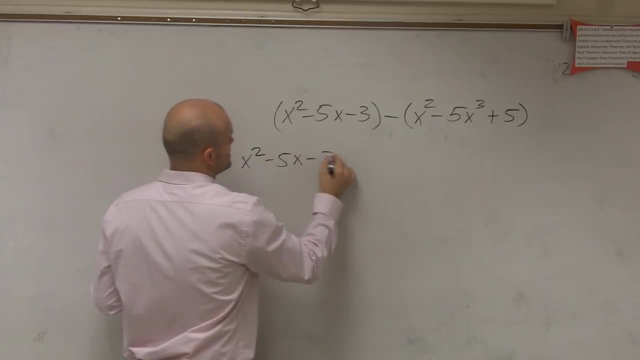 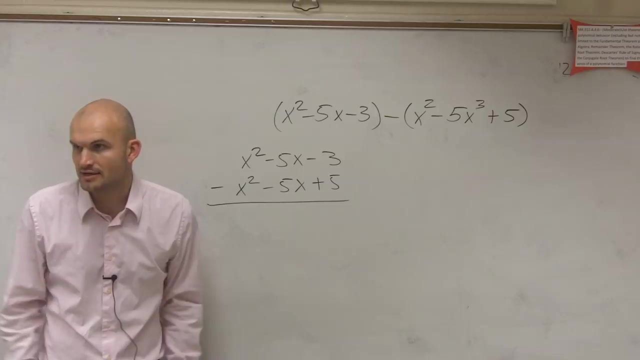 subtract. So you write x squared minus 5x minus 3 minus, and then you have x squared minus 5x plus 5.. Now I like this method because it's pretty simplistic. All you do is you take one equation and then you put it under the other equation and you subtract them. 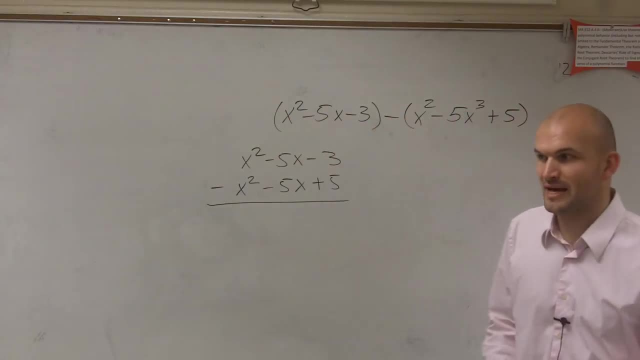 right. It's pretty straightforward, pretty basic. I don't like this method because a lot of times students make get mistakes and they forget that you're subtracting this whole bottom equation from the top, or this whole bottom polynomial from the top polynomial. 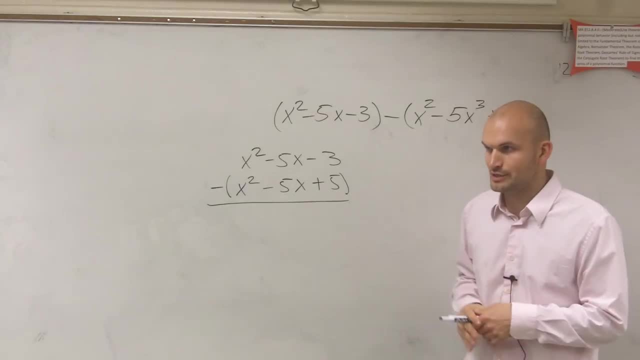 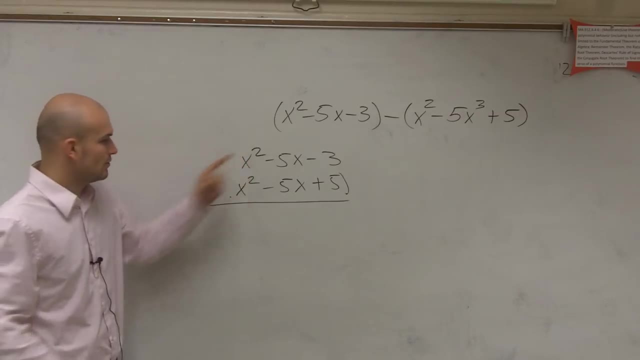 So when you do this, you have to kind of say it out loud to really make sure you're doing the correct operations. all right, So here's how I'm going to help you. So I have x squared minus x squared, which is going to be yes. Oh, that's not supposed to be a 3, I'm sorry. 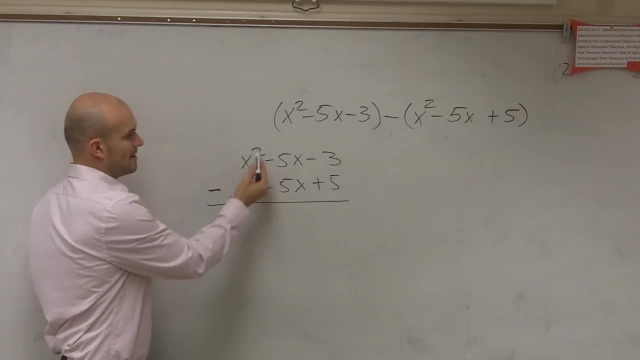 that's supposed to be an x, sorry, Okay. so x squared minus x squared is 0x squared 0 times x squared is just going to leave us with 0, right. So now? negative 5x minus negative 5x. Remember, those are double negatives, so it's going to be negative 5x minus negative. 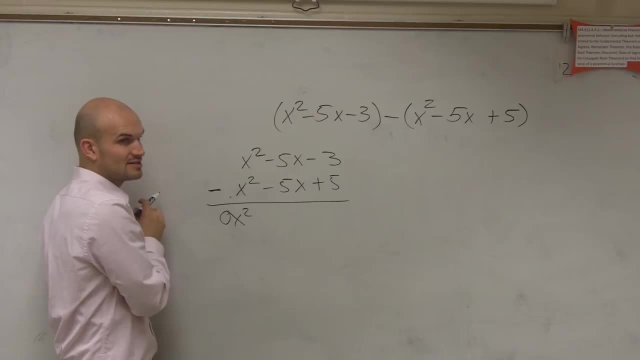 5x and it's going to turn to positive. so therefore, negative 5x plus 5x is going to leave us with 0x, and then we have negative 3 minus 5, which is just going to leave us. 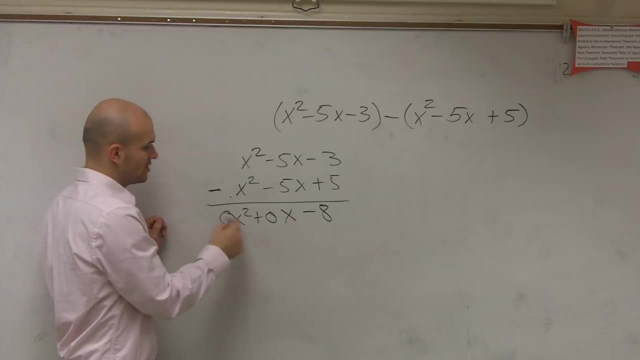 with a negative 8.. Well, obviously, like I said, these are all going to multiply to give you 0, therefore, your final answer is just going to be negative 8 in this example. okay, Cool. Now here's the other method that I think. 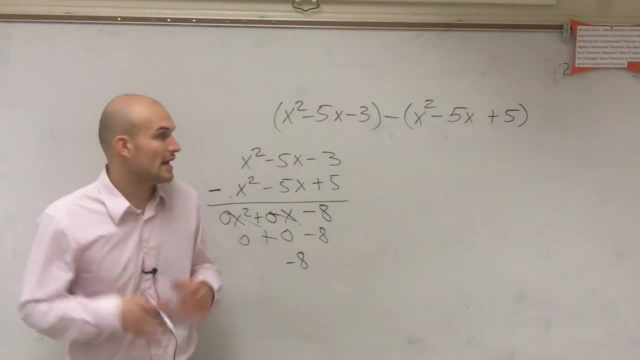 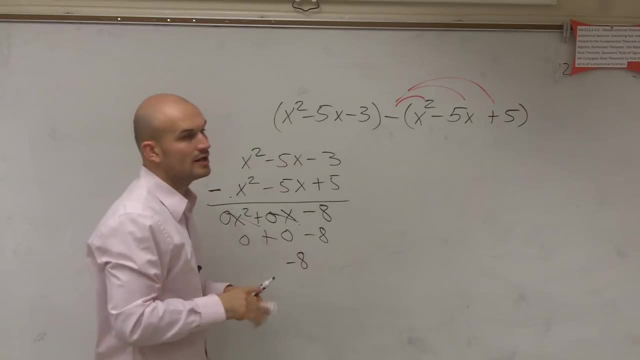 makes it a little bit easier, because I really don't like doing subtraction like this. What I prefer to do is apply the distributive property with your negative symbol. okay, Therefore, and then remember, remember, guys, when you first learned adding and subtracting numbers.